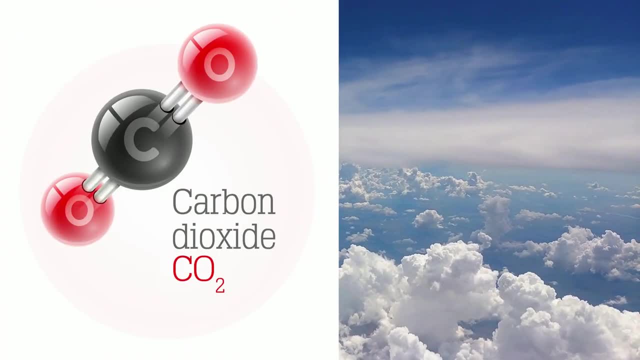 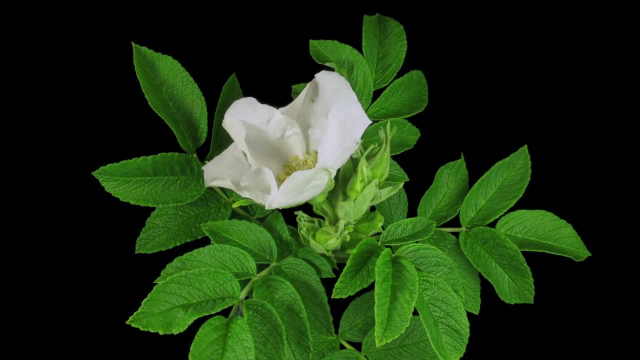 Carbon is found in the atmosphere in at least two forms: carbon dioxide and methane. This atmospheric carbon can be absorbed by autotrophs like plants and plankton to be used for photosynthesis. It can also be absorbed by bodies of water and the ocean. 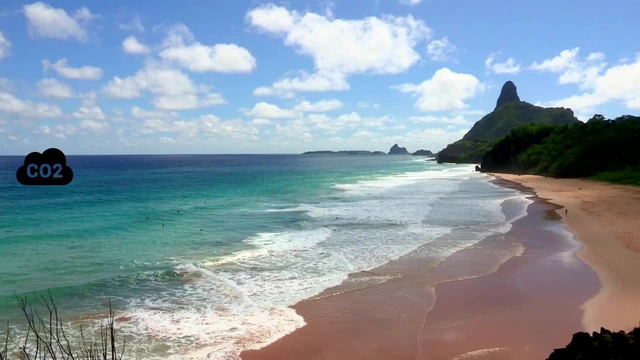 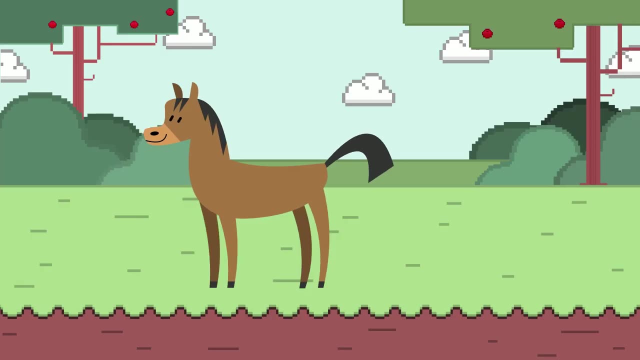 When carbon is absorbed by the ocean, it reacts with the water and creates carbonic acid. The terrestrial biosphere, which is another term for the earth's land, has several paths of carbon that it can take. First, there is an exchange between plants and 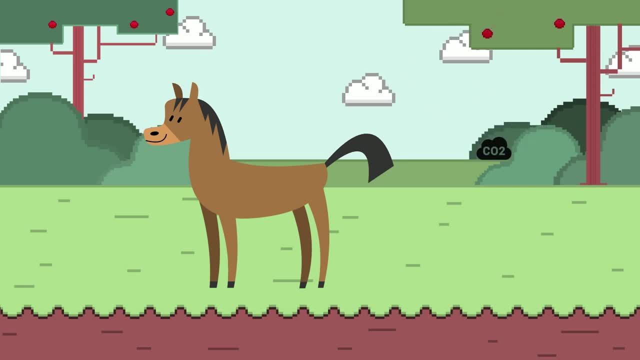 animals. Plants absorb carbon in the form of carbon dioxide for photosynthesis, and animals release carbon dioxide during cellular respiration. Also, heterotrophs eat plants that contain carbon. Animals also release carbon as methane during digestion, And the soil contains decomposers that release carbon into the atmosphere and the soil. 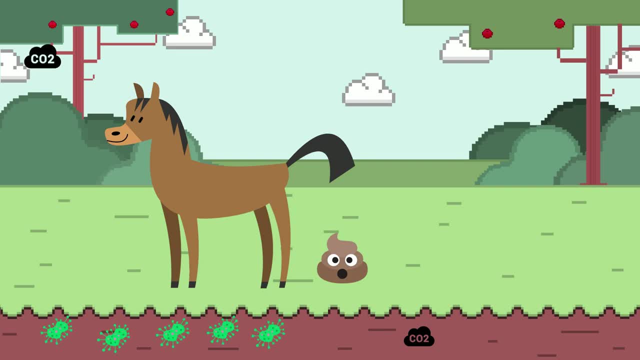 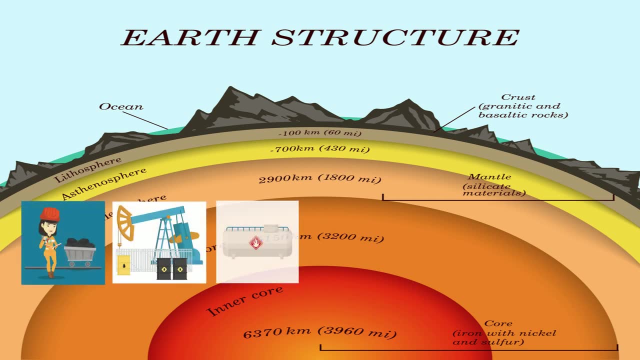 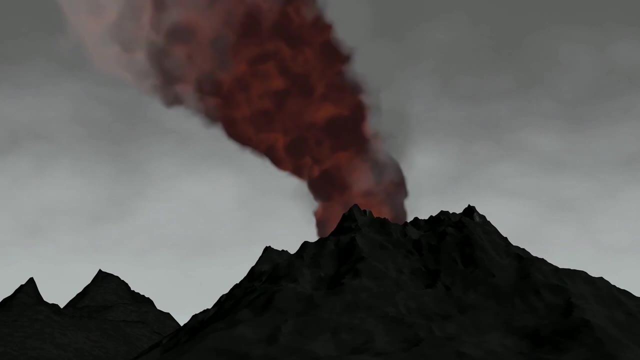 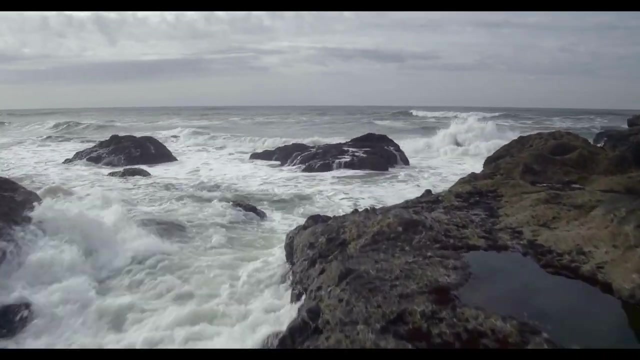 Carbon is also stored in the Earth's interior. Carbon in the lithosphere includes fossil fuels like coal, oil and natural gas, along with deposits like limestone. And volcanoes may release some of this carbon stored in the lithosphere when they erupt up. next, the ocean. the ocean has the greatest exchange quantity of cycled carbon and stores 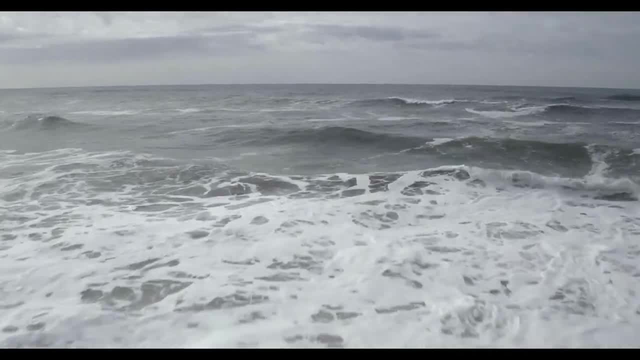 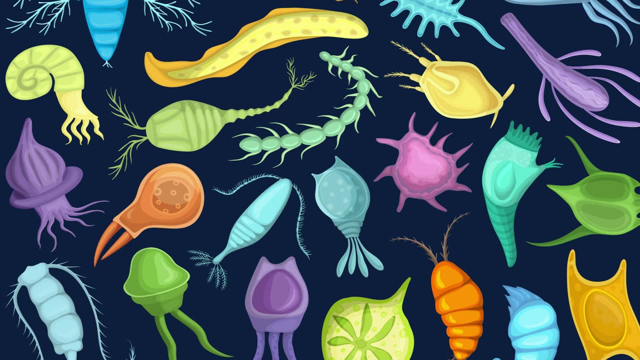 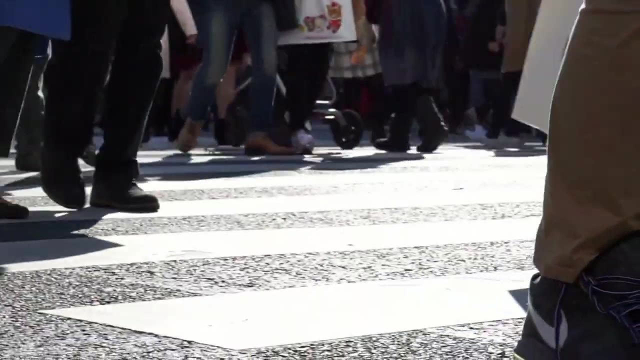 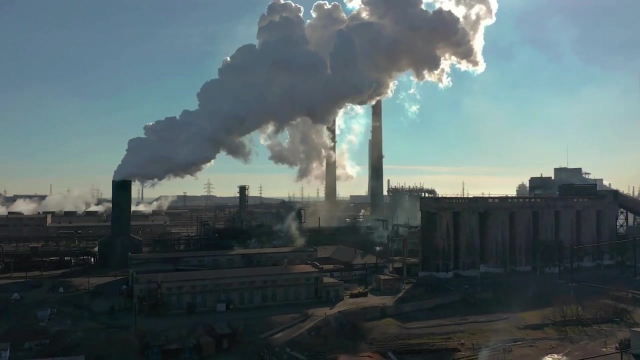 a large amount of carbon. the ocean absorbs carbon in the form of carbon dioxide. the ocean. ocean also has a large amount of plankton that absorbs carbon dioxide that it uses for photosynthesis. humans also influence the movement of carbon. humans burn fossil fuel, which releases carbon dioxide into the atmosphere. also the production of clinker, which is used for cement, from limestone. 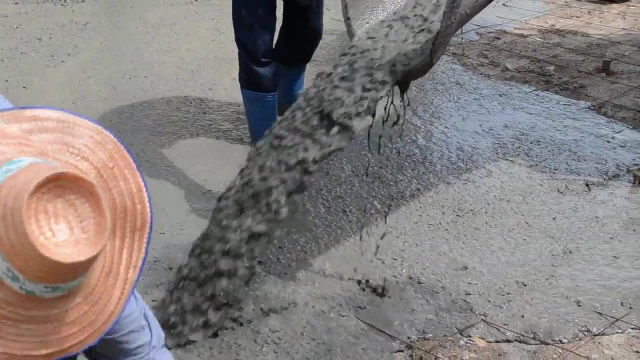 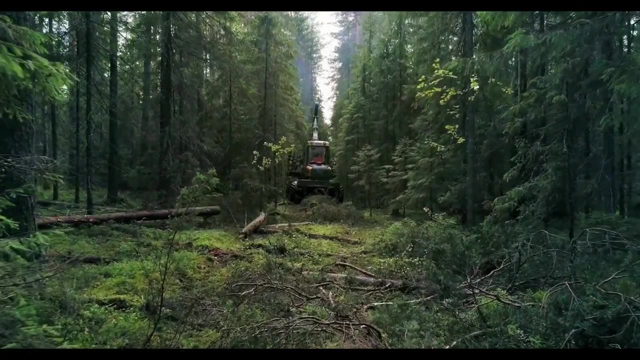 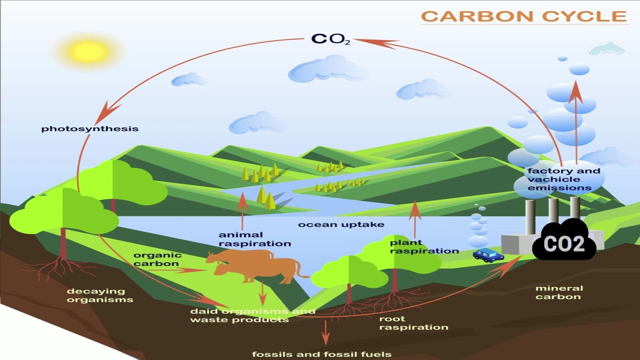 also releases carbon. in addition, deforestation from humans can cause the amount of carbon in the atmosphere to increase. so there you go: an overview of the path of an atom of carbon that may take place during the carbon cycle. thanks for watching. and moon math uploads a new math. 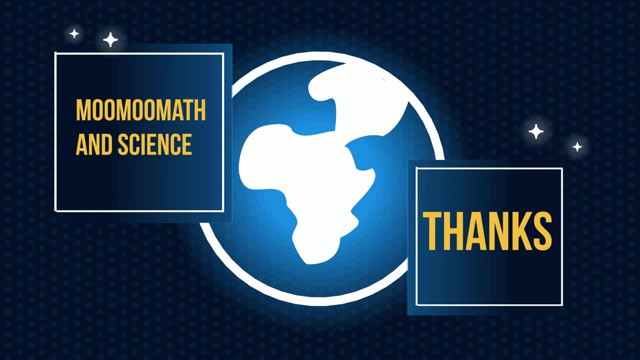 and science video every day. please subscribe and share.